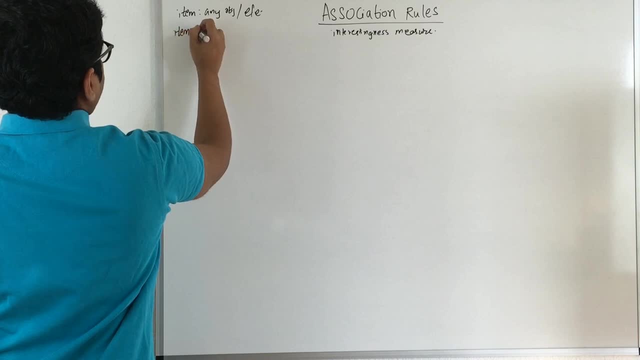 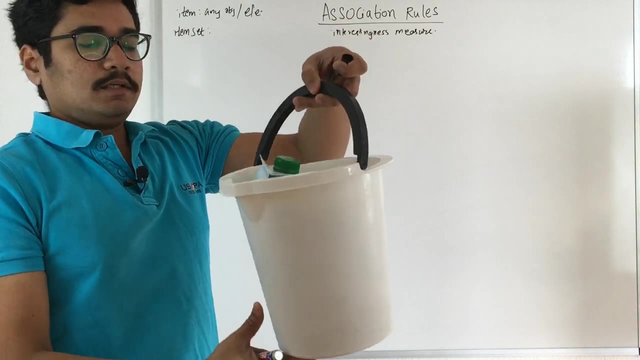 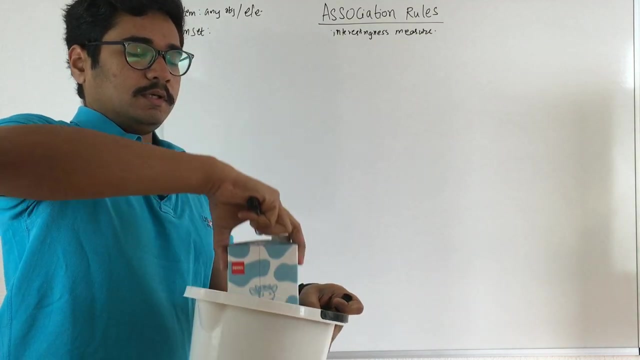 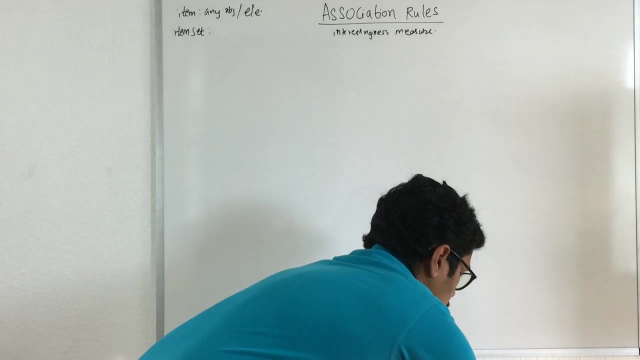 any object or element. No, What is an item set? Item said, Say: I have a basket And it contains contains one juice and one milk. So these are two items that are frequently occurring. So in the real world, its collection of one or more items, that is item set. 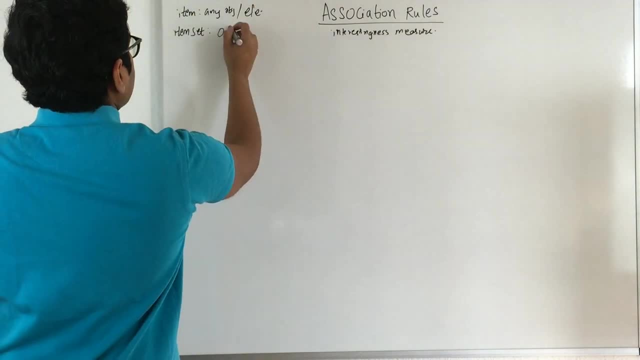 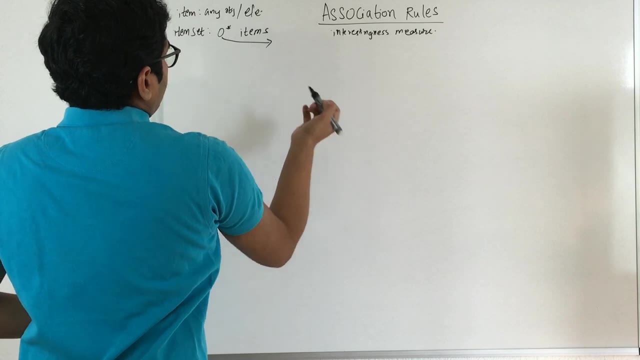 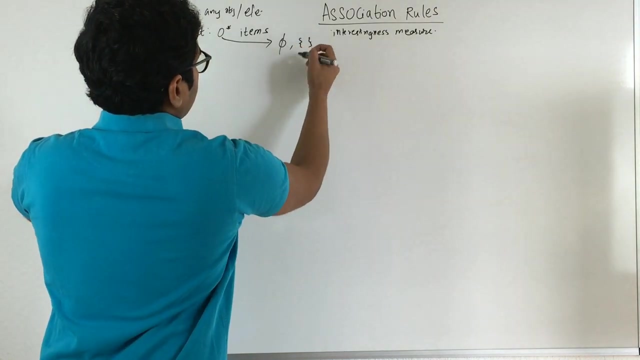 But when you define association rules, it becomes zero or more items, collection of zero or more items. And so why this zero? Because if there are no items present, so you consider this fee that is empty set, or it's also done as this one, or it is the null. 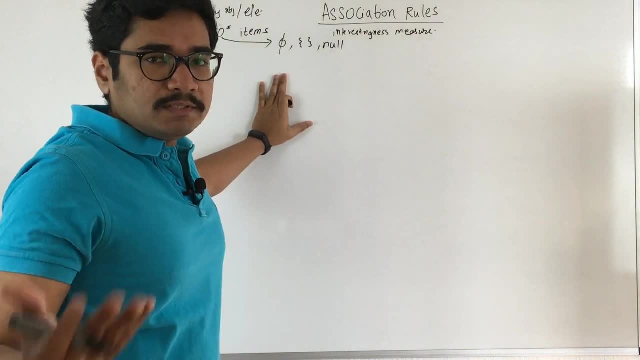 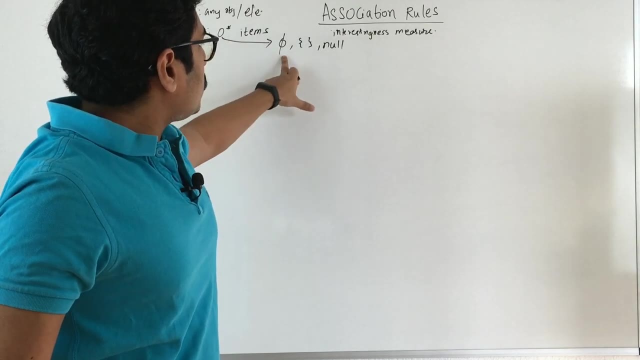 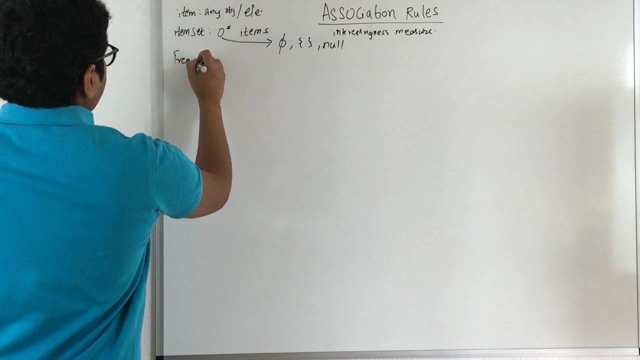 So whenever you construct an item set like this, so we'll be seeing in our future videos, So there will be considering this zero item. So this is zero stands for either fee or this empty set or null set. Next, what you have is called as frequent item set. 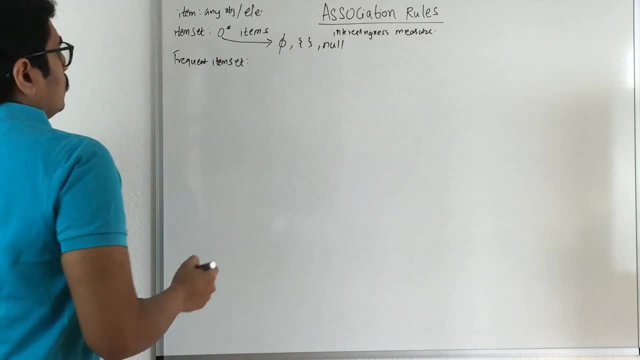 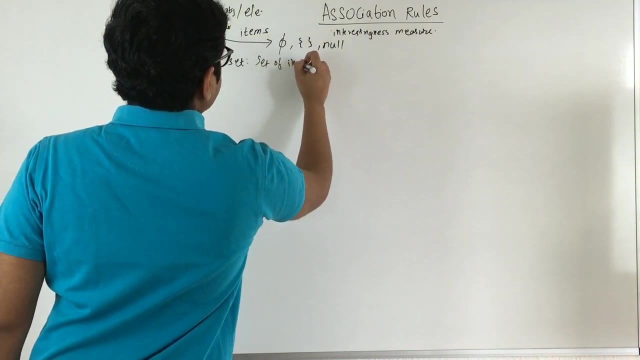 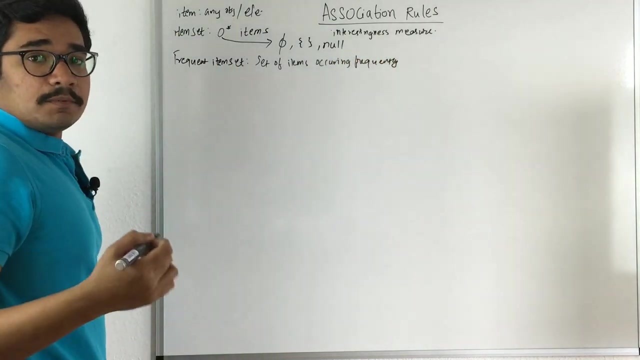 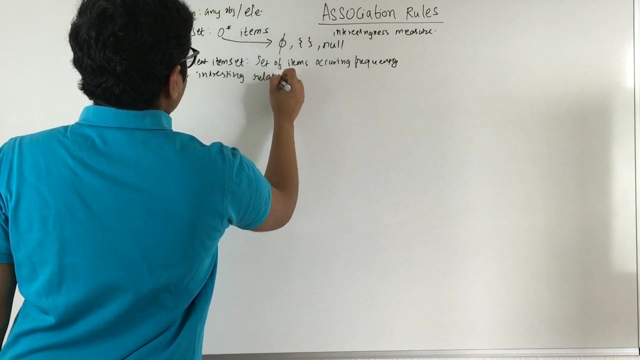 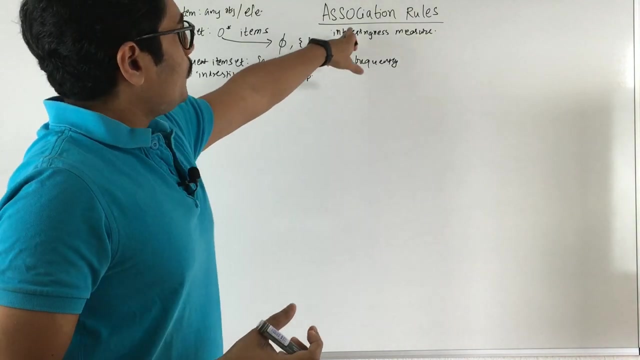 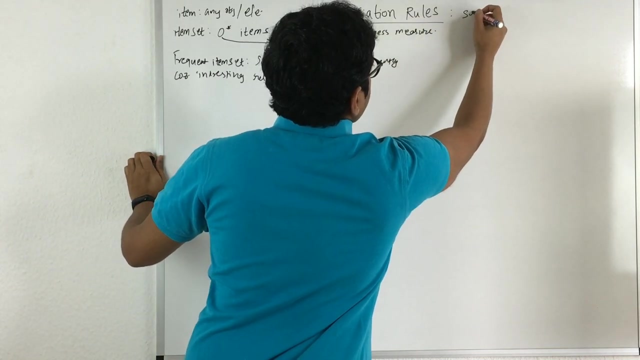 Okay, Which is set of items that are occurring more frequently. Frequently why? because they have some interesting relationship. And so if you want to identify or extract that interesting relationship, We define association rule. so association rules can be used to say as set of interesting. 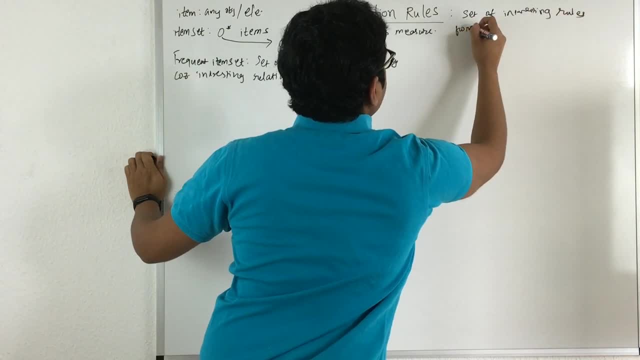 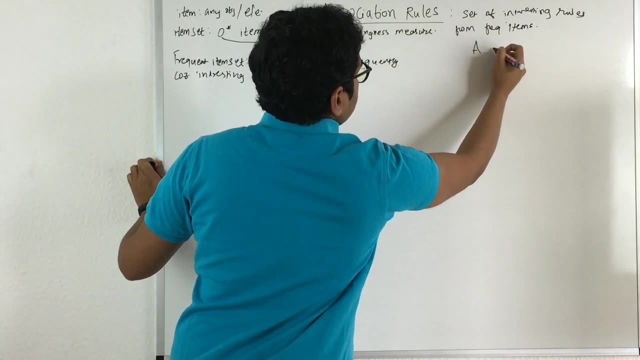 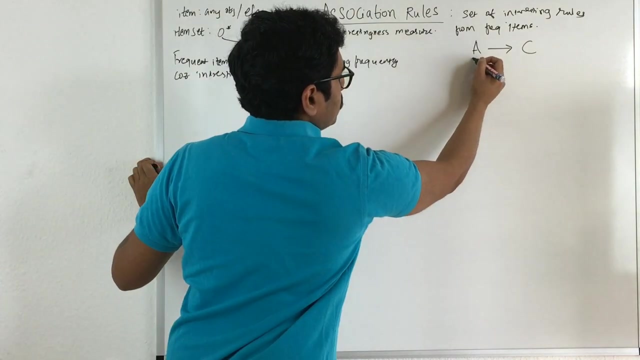 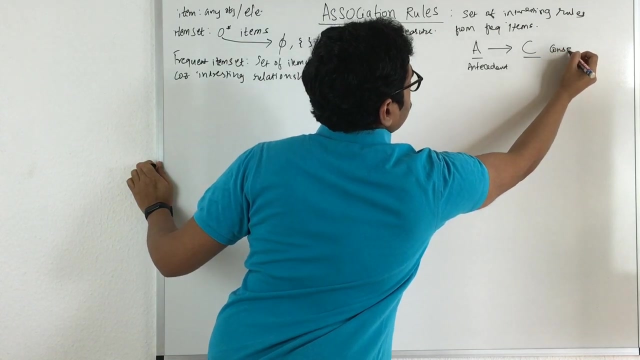 rules from frequent items, And so it is represented as this way. So whatever items or item set is present on the left-hand side, or whatever See here, this is called as the antecedent and this part is called as the consequent. 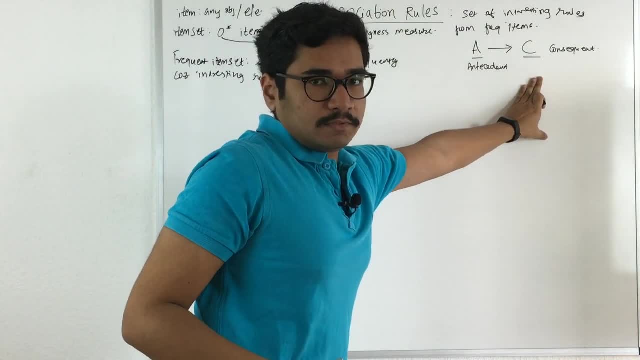 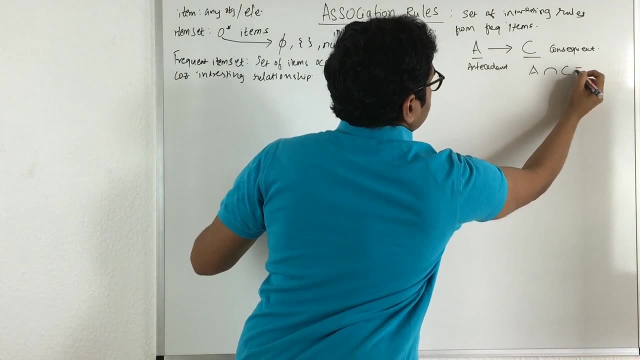 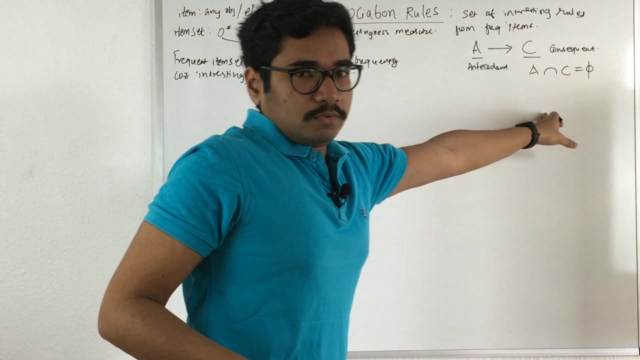 So as a result of this item set, you derive this, so it's written in this way. So in terms of crisp set theory, you have a intersect. C is equal to phi. that is disjoint. That means there are no duplicate or redundant items present in both of this. 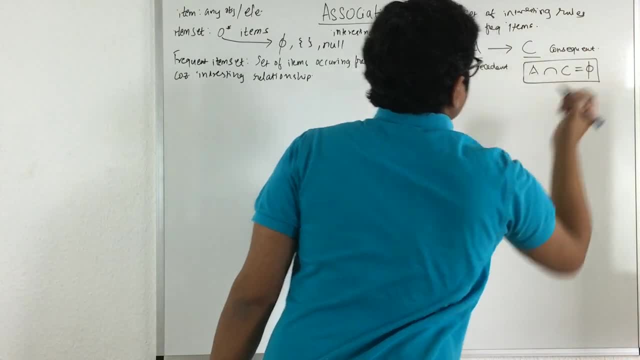 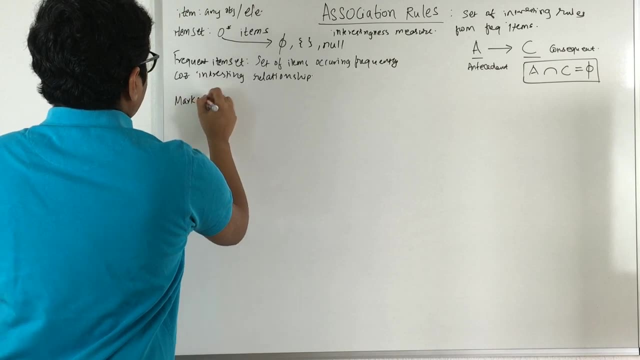 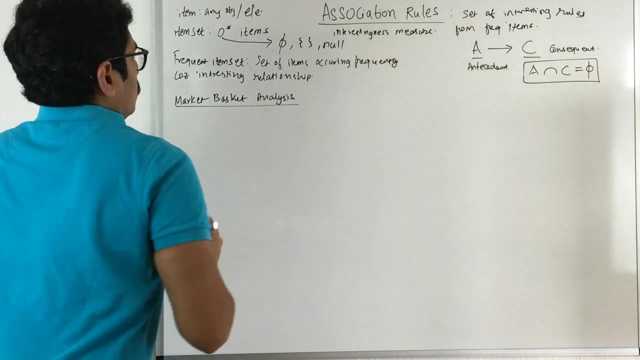 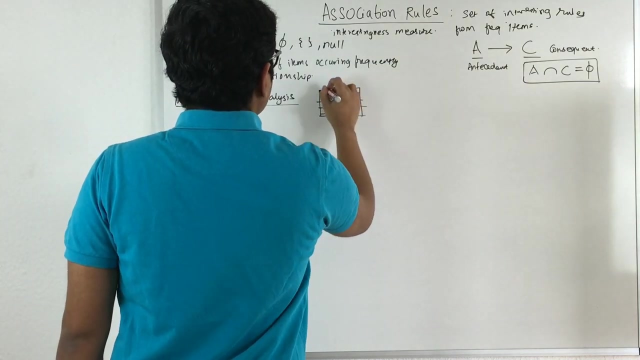 So this is the condition that is satisfied By Association rules. Now what you need to understand is something called as market basket analysis, So you know the relational DBMS, that is, you have something like this: You have rows and columns, So there, this particular row, this was called as tuple. 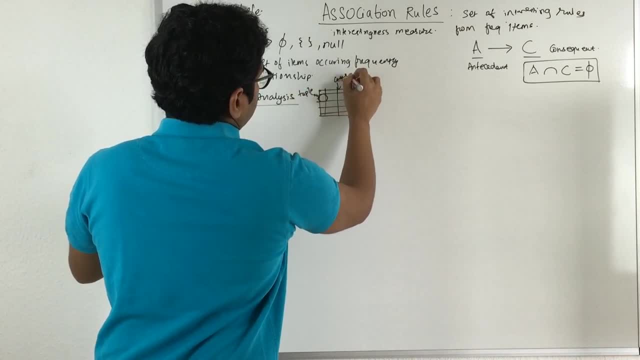 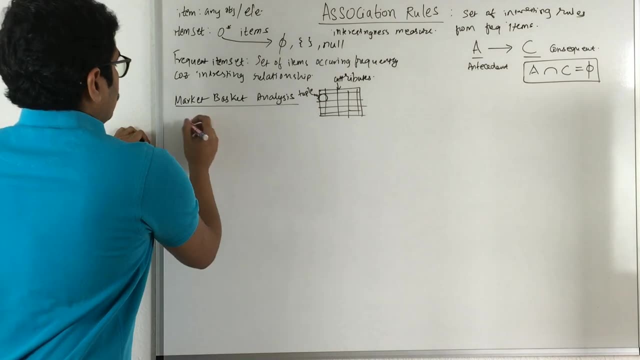 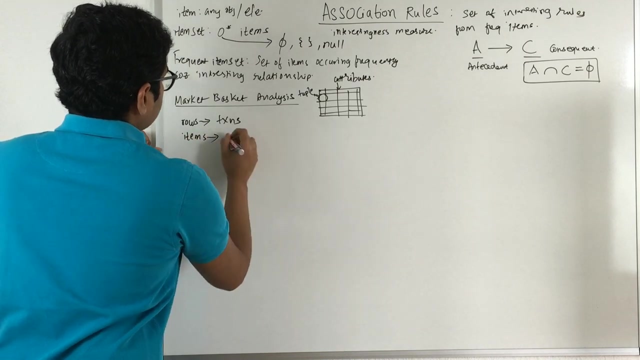 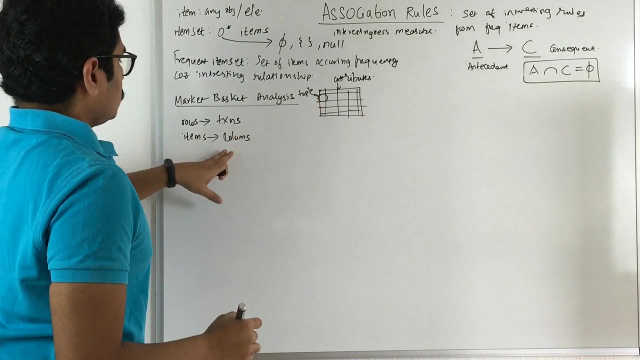 And this was called as the attributes. But when you deal with association rules or frequent item set, mining this, rows are called as transactions and items are called, as that is, the columns, transactions as the rows and items in the columns. So you can also represent this in an asymmetric. 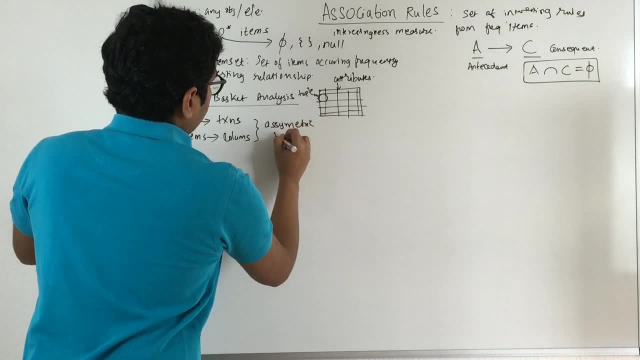 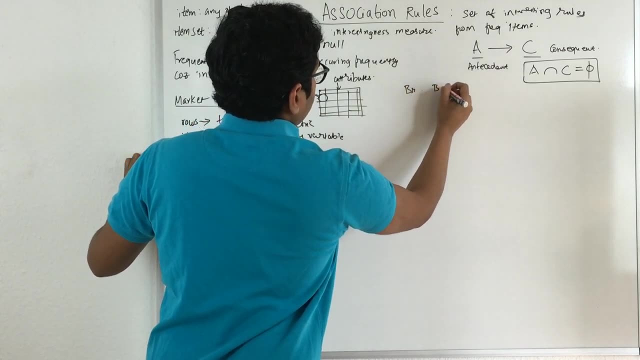 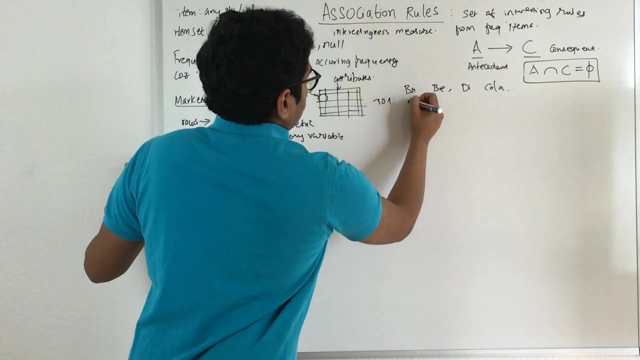 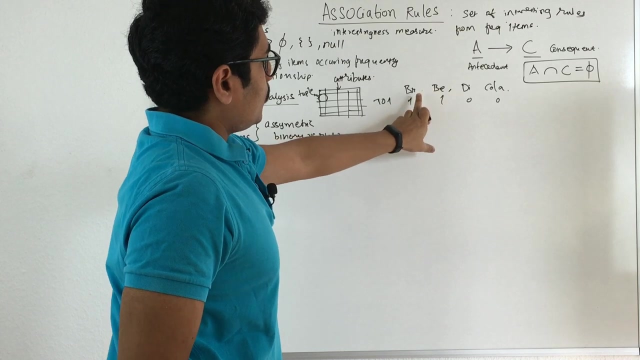 Asymmetric binary variable. So say you have bread, then beer, then you have diapers and Cola. So say you have first transaction. so you can represent like this means in the first transaction beer is consumed, bread is consumed, beer is consumed, but no diapers or no Cola is consumed. 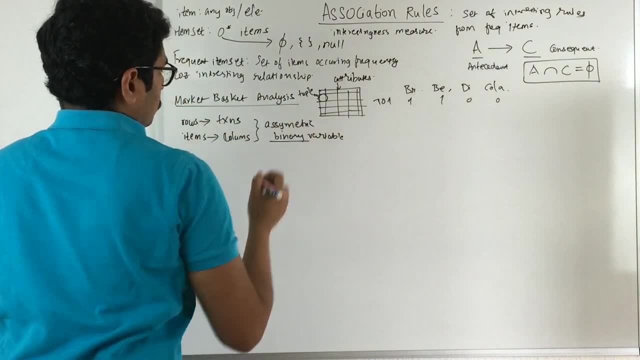 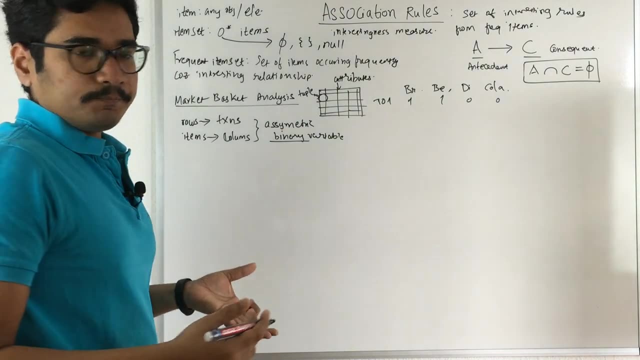 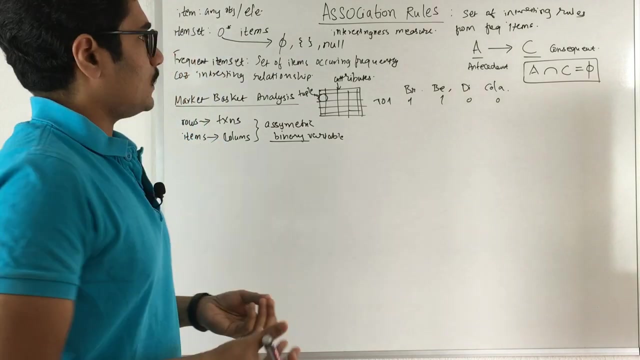 So you have binary representation, So that is a binary variable. Now what you need to do is you have such kind of market basket. So from this market basket you need to analyze certain different patterns, or frequency of different patterns occurring, with the help of association rules. 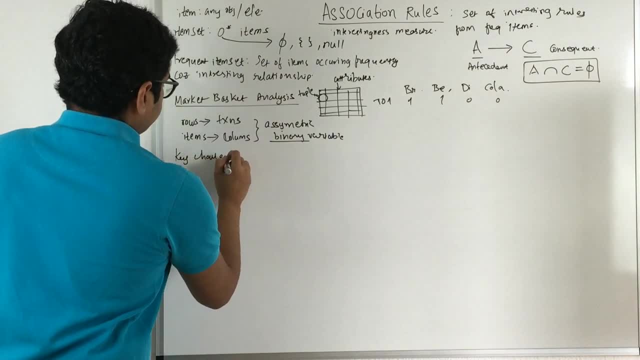 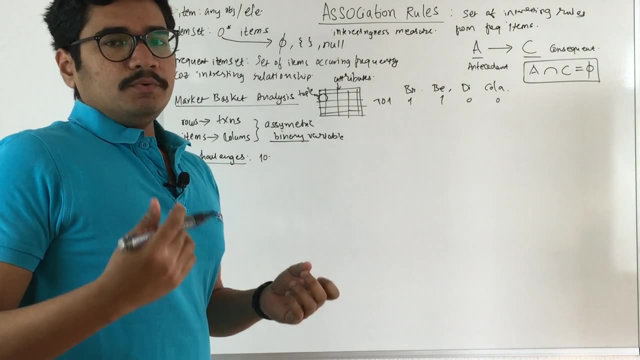 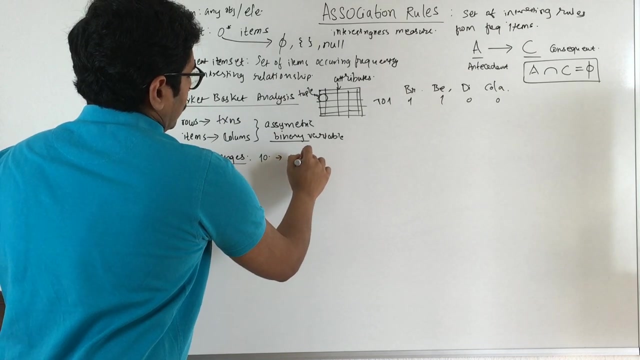 So there are some key challenges to this. To market basket analysis, Say you have set of 10 transactions And you need to apply this association to it, So that's not a big difficulty in doing. but instead, instead of this 10, you have 10 K or 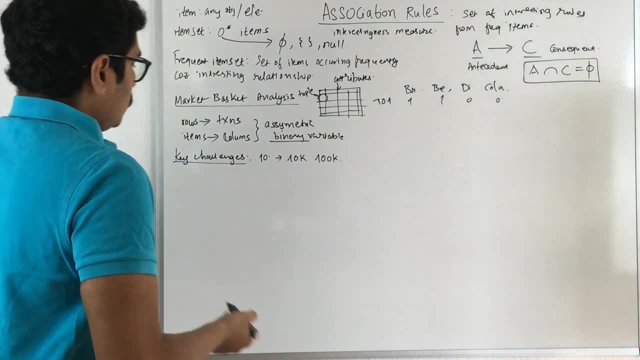 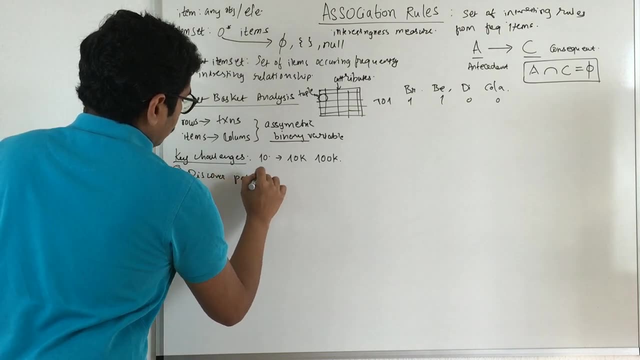 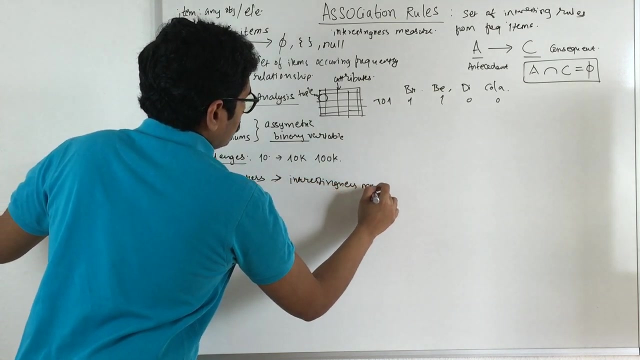 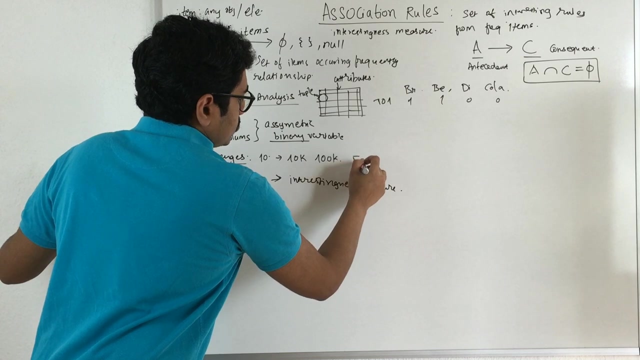 100 K number of transactions and it becomes very difficult. So you need to first challenges, you need to discover patterns which has some interesting as measure. So let's say, by any means, By any means, You have discovered this patterns and out of this, 50% of the patterns are valid and 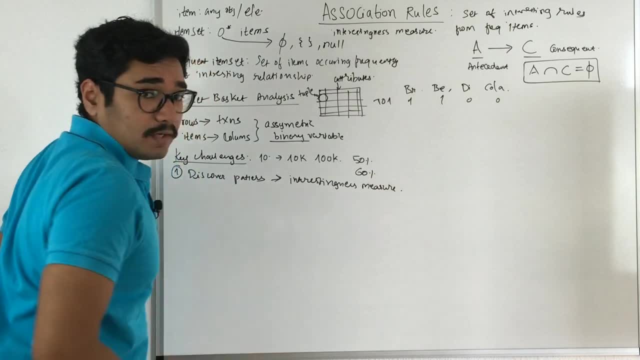 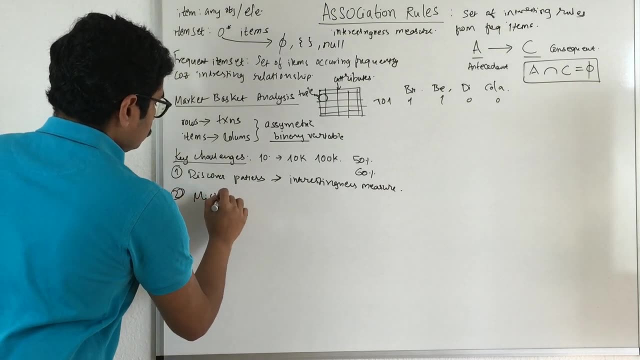 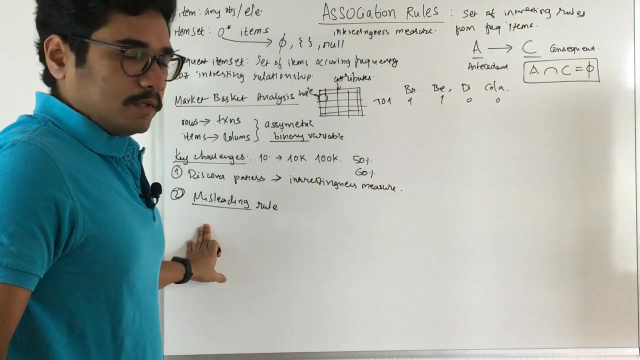 50 are not, or it can be like 60% of the patterns are invalid. So it can also happen that there are some misleading rules. Just focus on the word misleading, because we'll be encountering this word in the future topics, So misleading rules will carry some spurious information. 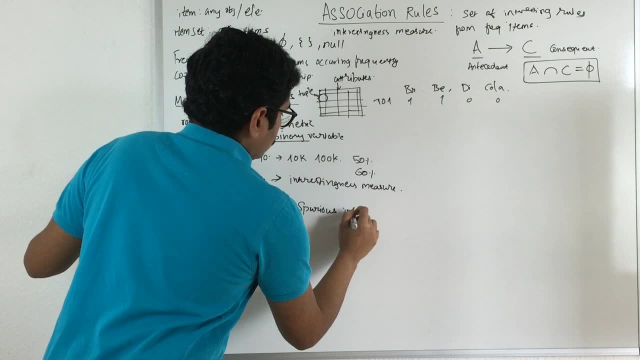 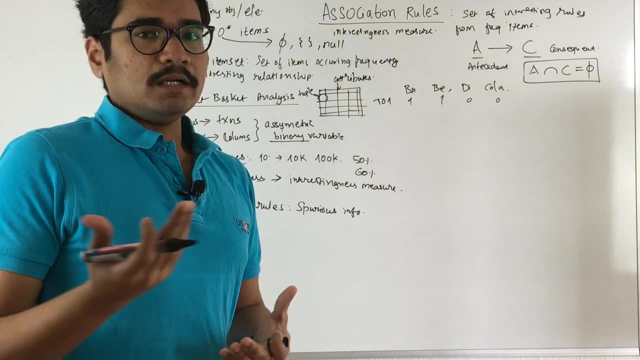 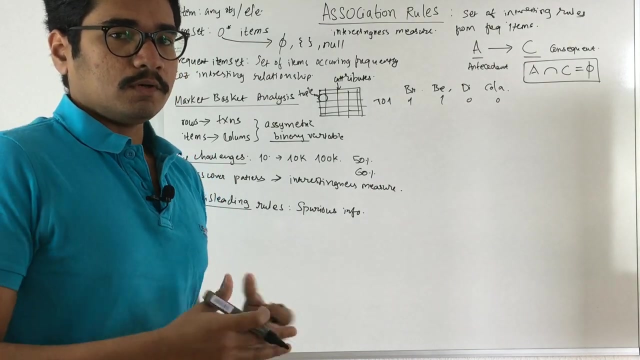 So misleading rules will carry some spurious information. So misleading rules will carry some spurious information. That means it's kind of fake or false information which will lead to some inconsistent or unreliable results. So there, you need to have some kind of measure or some kind of rules in order to eliminate. 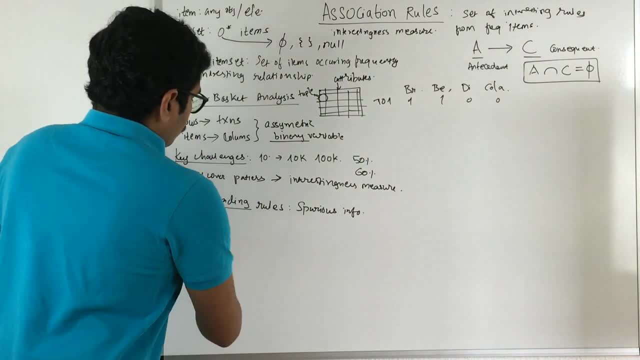 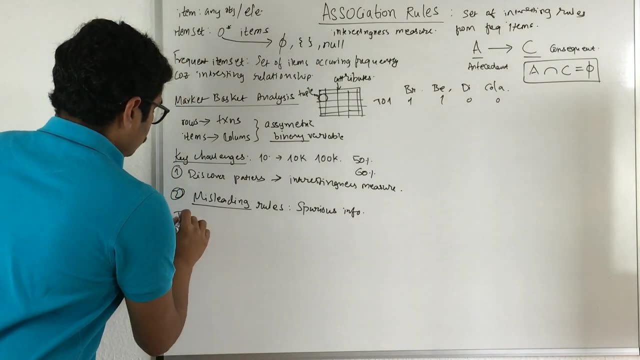 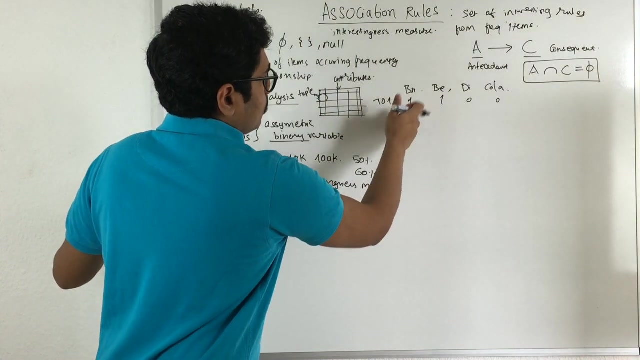 this kind of things. So we have these two challenges for market basket analysis. Next, what we have is we have transaction. So one particular transaction, Say one customer went to a supermarket and he took bread, beer, diapers and Cola and then he did his billing. 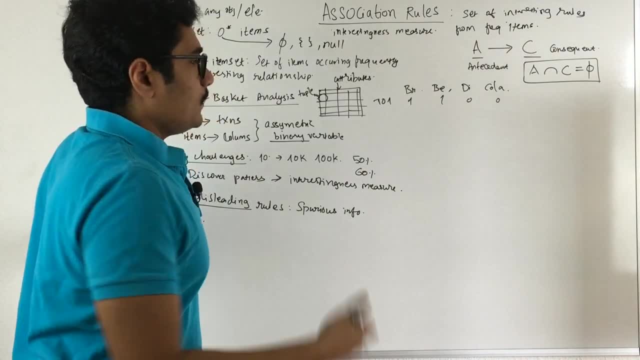 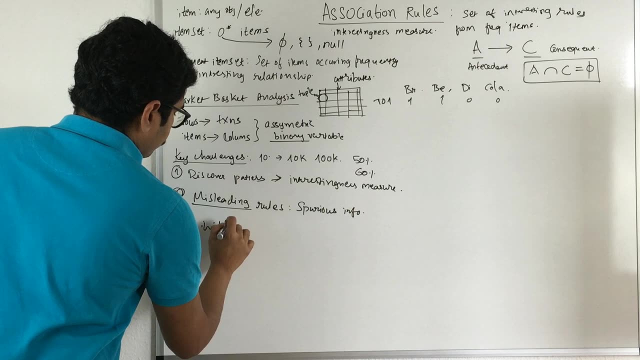 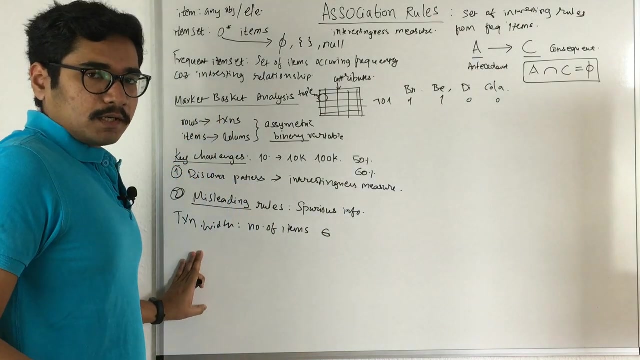 So that is one particular transaction. Similarly, second customer will come, he'll do another transaction. So likewise you have a set of transactions. So what does a transaction with? that is number of items that is contained or belongs to that particular transaction. that is transaction with. 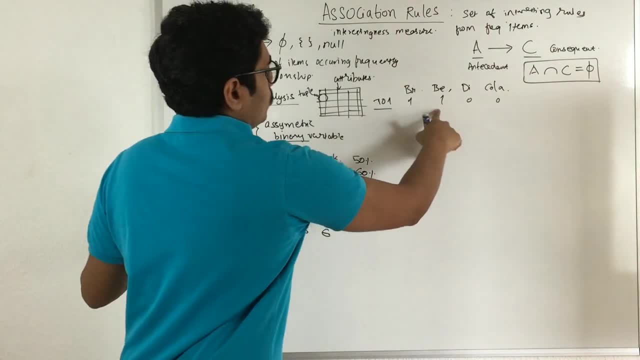 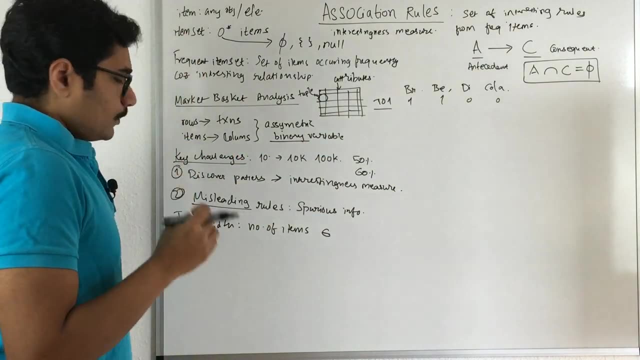 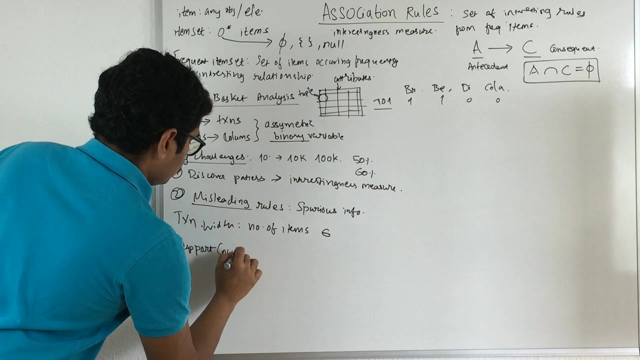 So if I ask you What is a transaction width of T 0- 1, you will say 1, 2, 3, 4, that is, 4 number of items are present in that particular transaction. Now, what do you need to understand is there is one term called as support count. 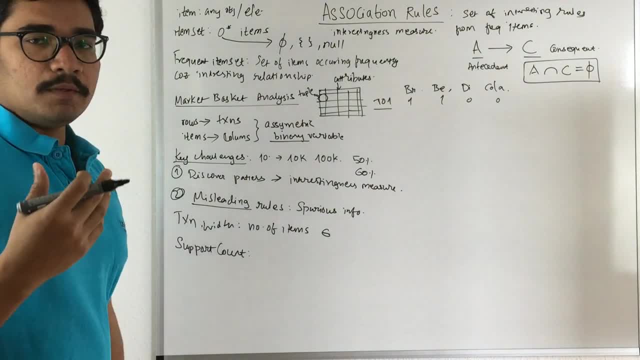 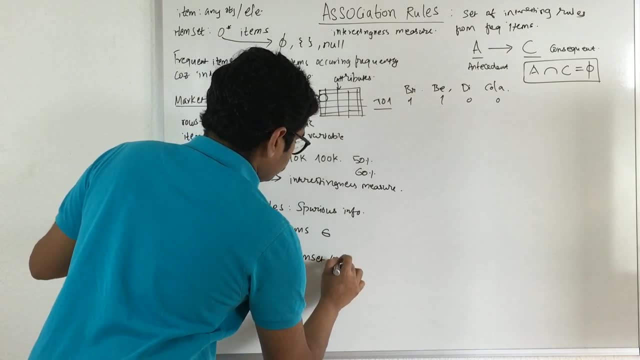 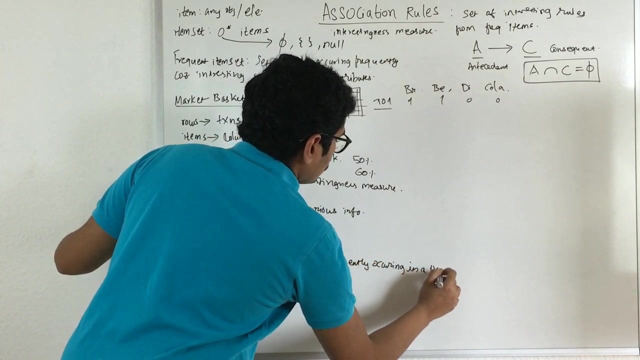 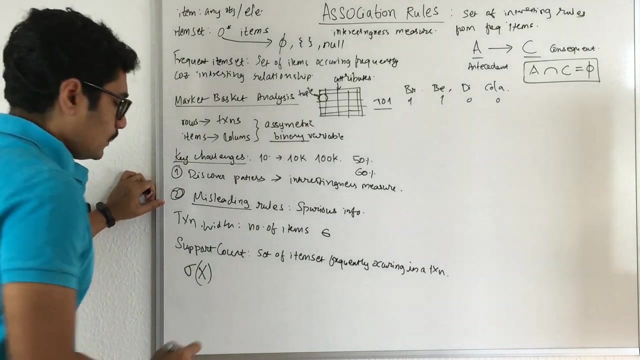 That is the set of item set that are frequently occurring in one particular transaction. Okay, That is the set of item set that are frequently occurring in a transaction, and so it is denoted by a symbol: Sigma and X represents an item set. Now, how do you define this mathematically? 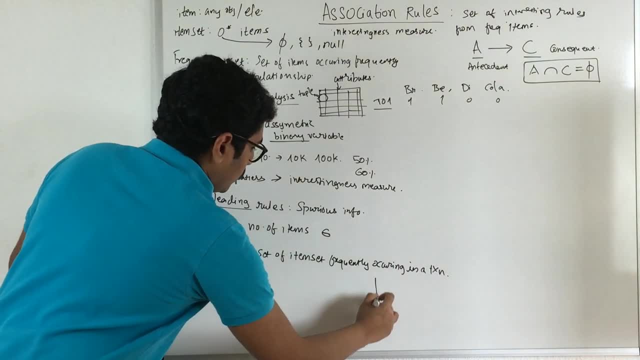 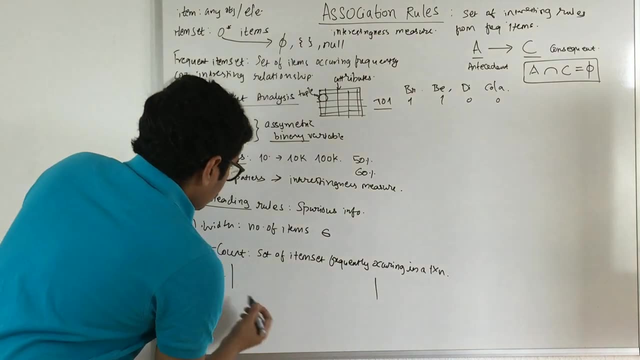 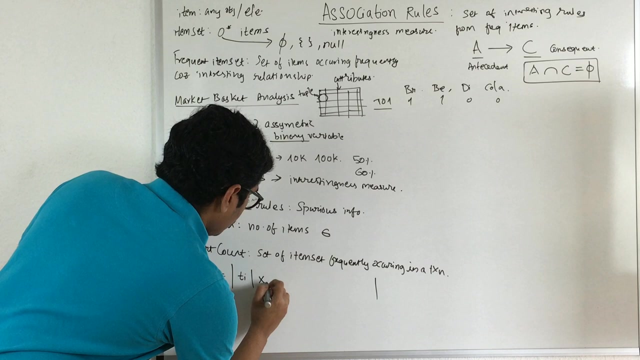 So this is a count, right. So you take a mod here means it should return an even number, not an even, but an integer. it cannot be negative. So you define this as Okay. So TI, that is one particular item, such that X is a subset of TI and TI belongs to T. 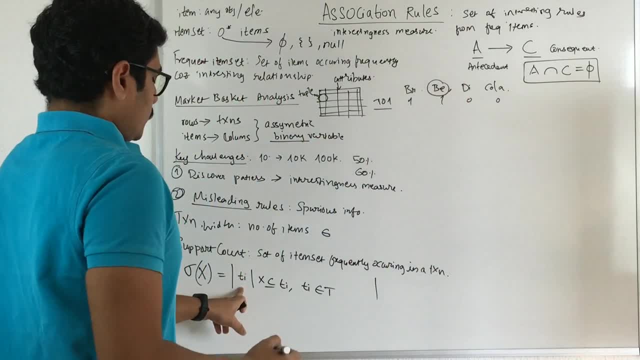 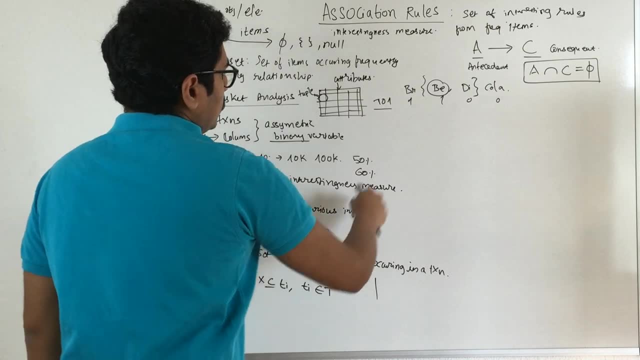 Now, if you just map this, TI is, you can consider beer, Suppose this is one particular item set- beer and diapers- so that belongs to this item set and TI belongs to one transaction. that is say, you have 10 transactions, T is equal to 10.. 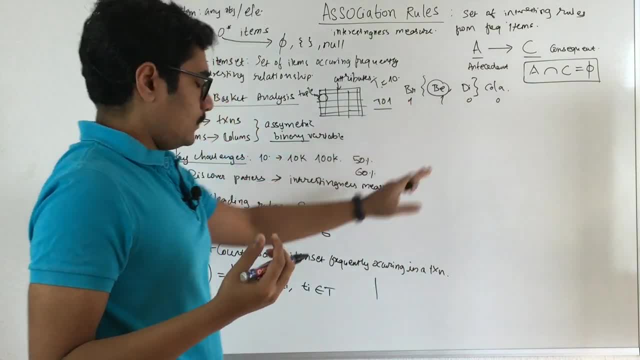 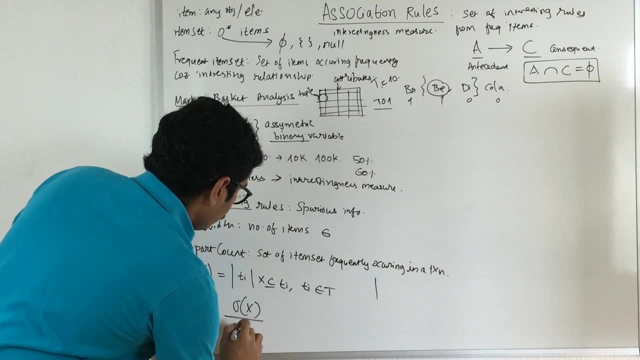 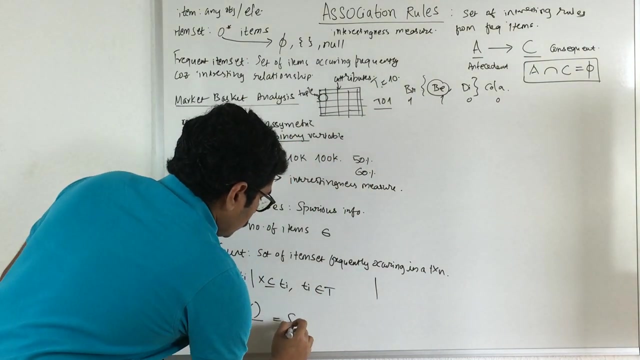 So out of this you have one particular transaction in that you have one particular item. So that is support count. and so when you divide this with the help of the total number of transactions- not the total number of items, total number of transactions- you get a measure. 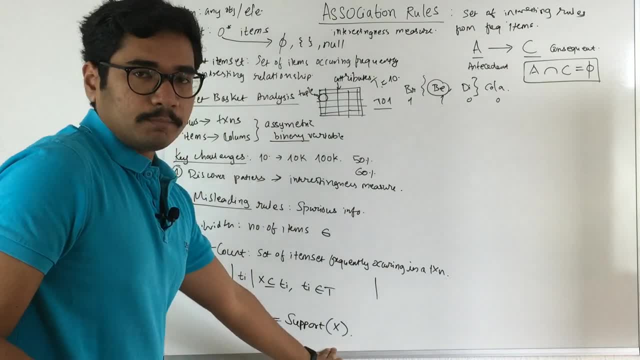 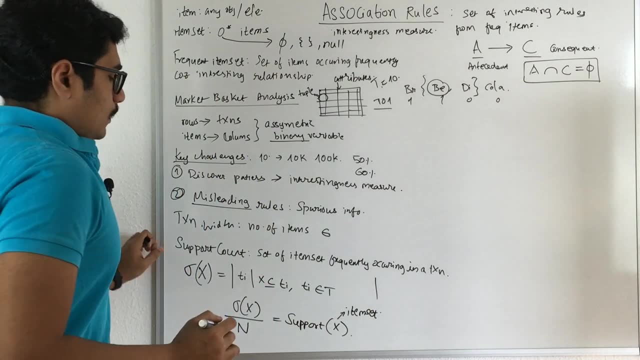 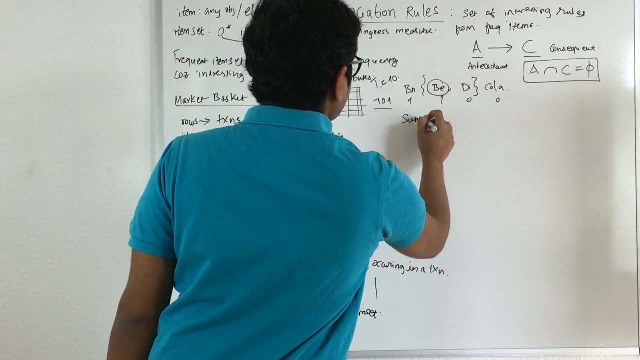 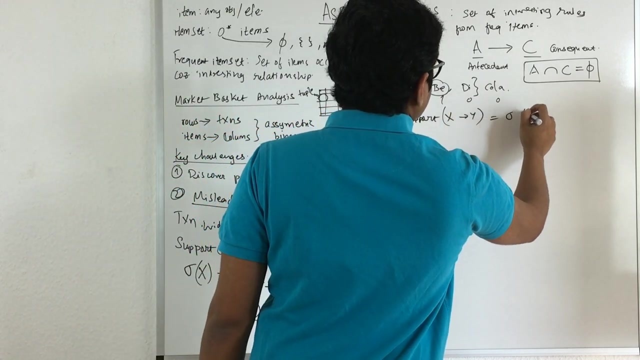 called as support. Now this is support over particular item set, that is X. X denotes item set. Now you can define X Or a support over a rule. also, Support over a rule, say X derives Y, So it is given as X union Y upon total number of transactions. 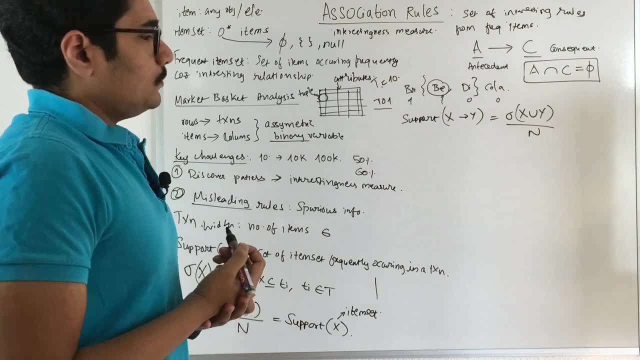 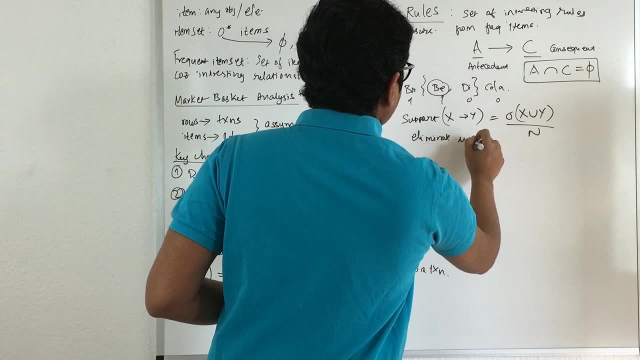 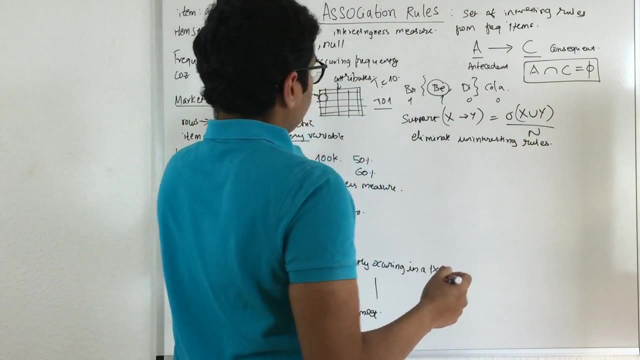 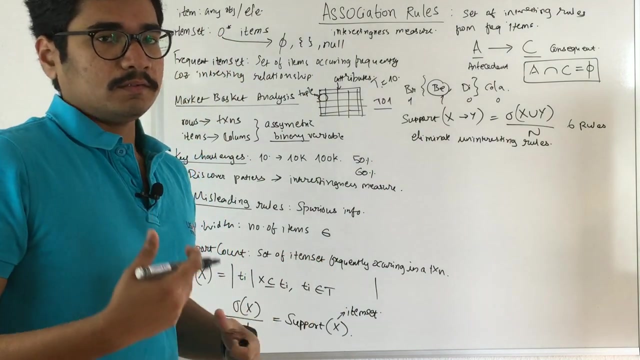 Now what support gives or what support is used for in association rule. So it is used to eliminate Uninteresting rules. So suppose in this particular transaction you have derived six rules in total and some of the rules may be redundant or some of the rules may not be that interesting to you. 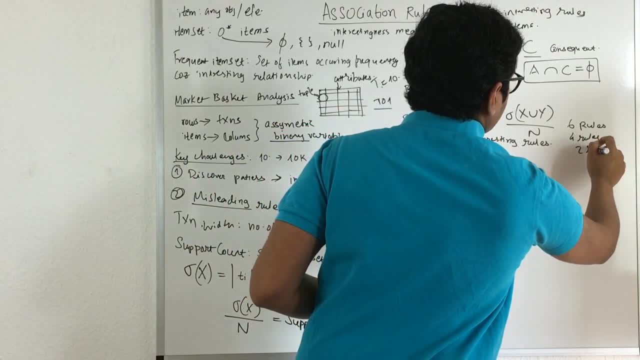 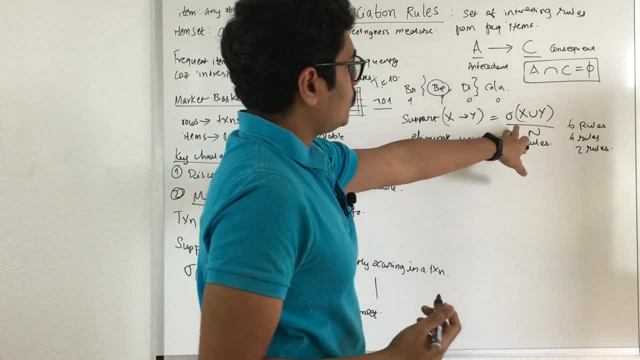 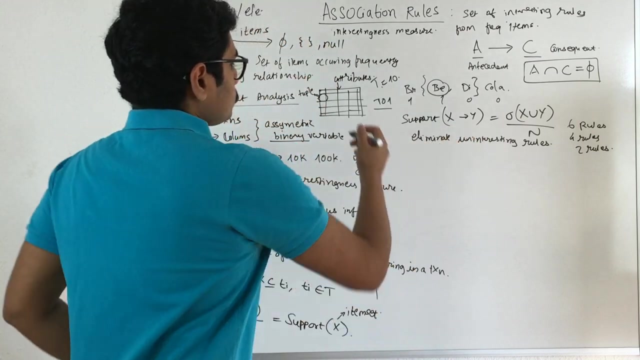 So you may have four rules or two rules. So support is used to eliminate such kind of things. so support, in mathematical terms, it's given in this way: As a ratio of X, As a ratio of X union Y, that is, the occurrence of these two events in a joint way, as a union. 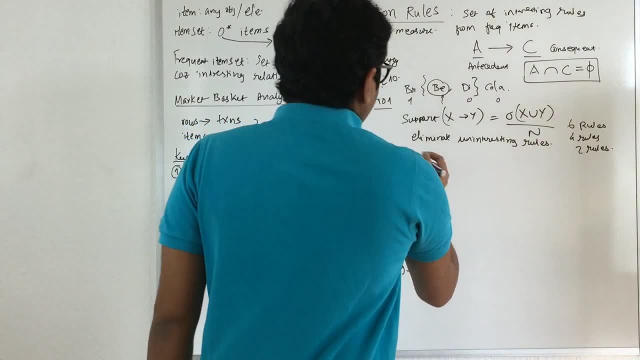 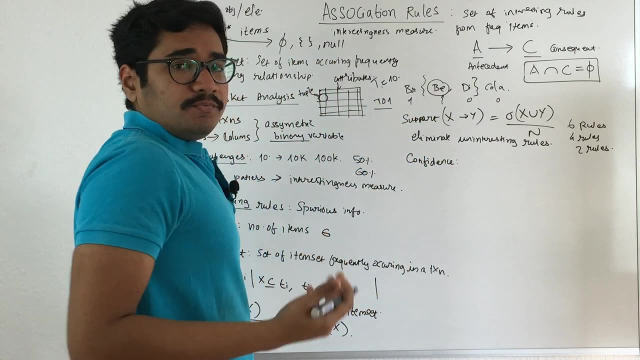 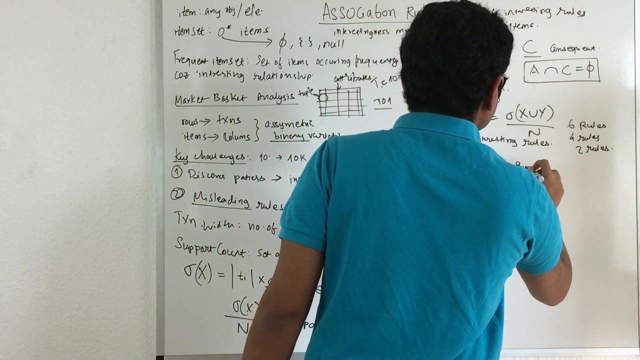 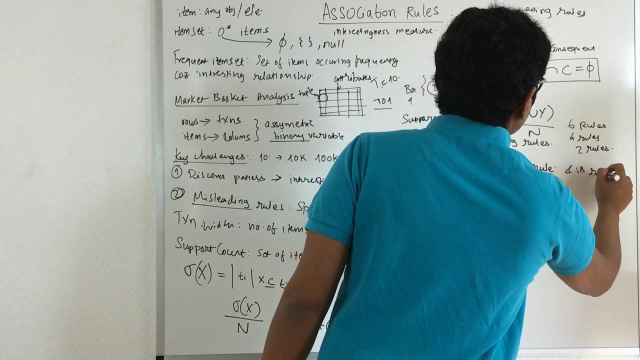 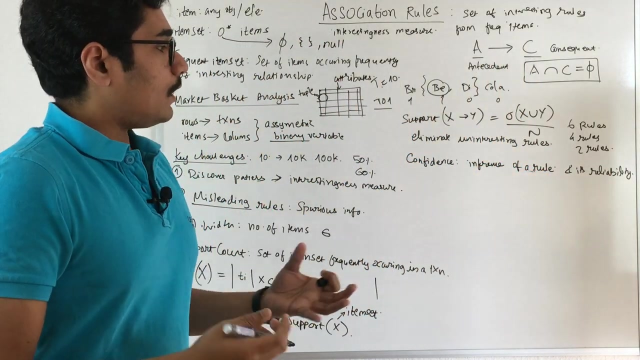 and divided by the total number of transactions, Next what you have is called as confidence. Confidence is defined as the inference made by a rule. Inference of a rule And its reliability Means you have got a particular rule. then how confident is that rule to apply to that? 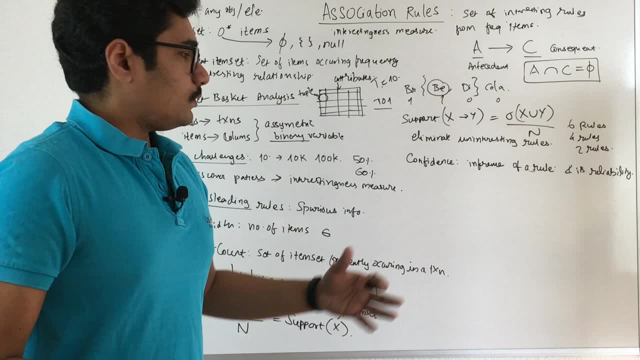 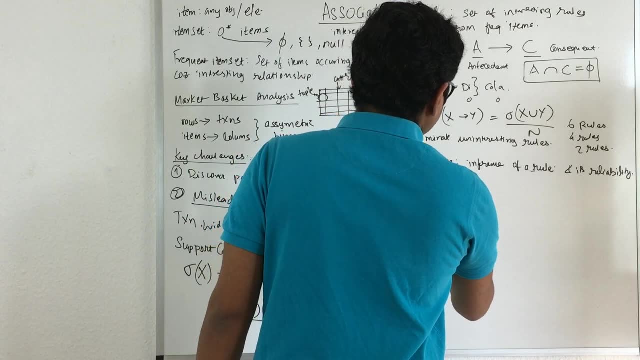 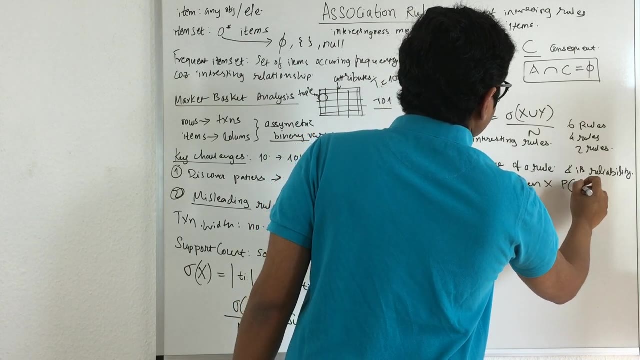 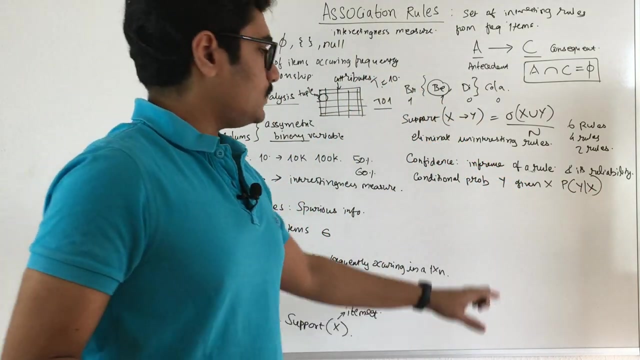 particular item set, Is it reliable or not? So that is defined by confidence. So confidence can also be written as the conditional probability Of Y given X, Confidence, Confidence. So this we have already seen in Bayes rule. So if you want to know what this conditional probability is, you can just watch that video. 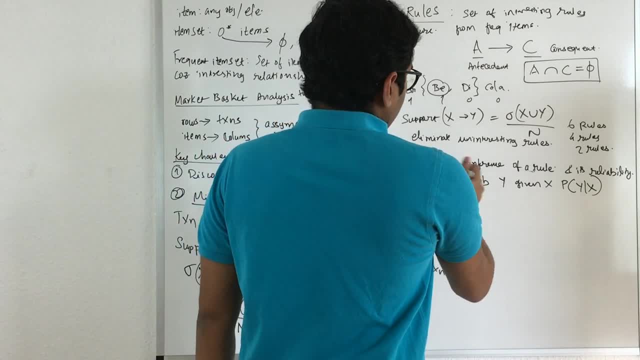 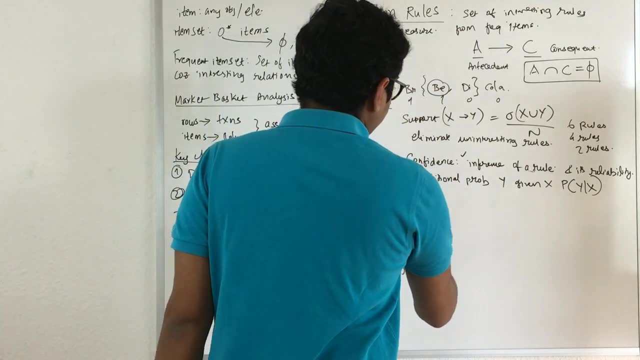 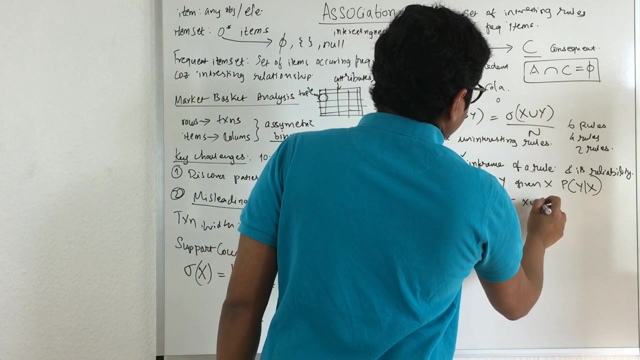 I'll give you a link in the description. So confidence is used to derive the inference made by a rule and it also defines the conditional probability. How do you estimate mathematically So confidence over a particular rule? X derives, Y is given as X, union Y upon whatever is there. 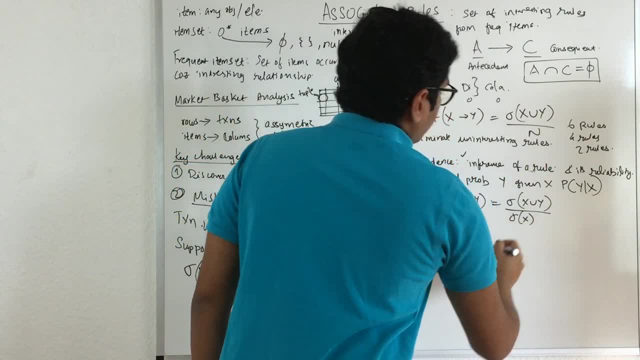 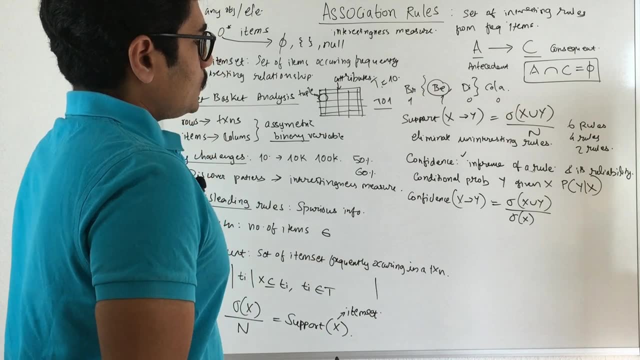 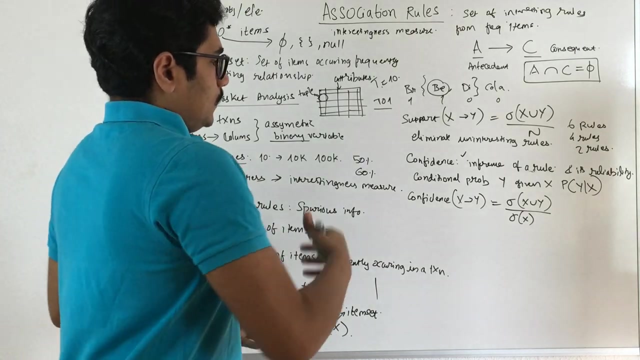 on the antecedent side. So that is Sigma X. So this is the confidence definition. Now what you have is called as the frequent item set. We have seen here that is a frequent item set. So how do you derive frequent item set? So in particular transaction you will: 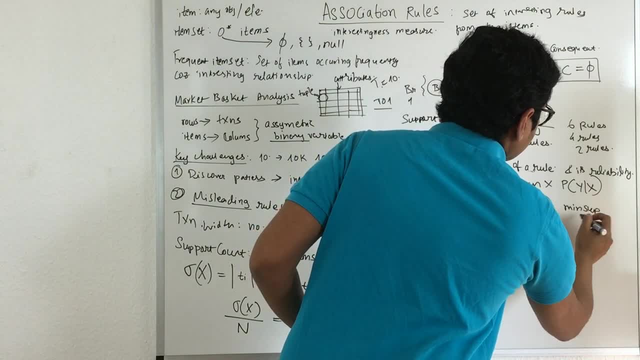 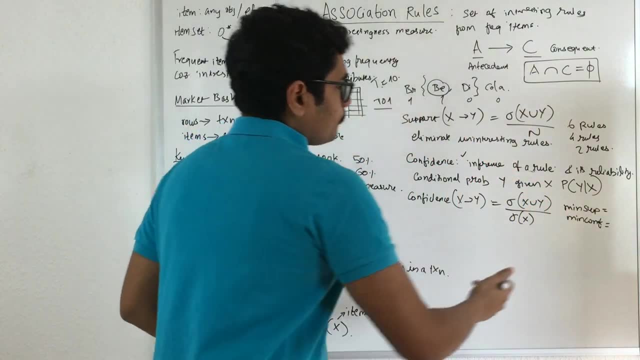 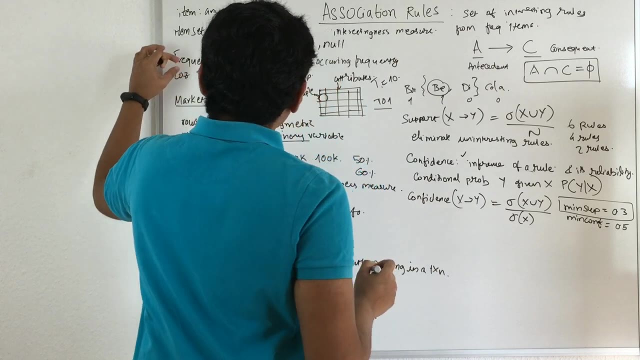 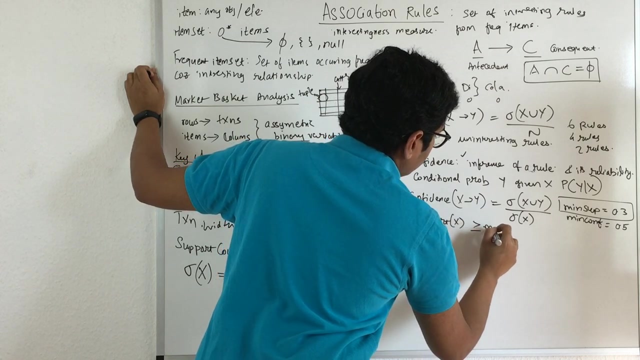 have some kind of parameter called as min sup or min confidence. So that is given by the mining algorithm. So say you have 0.3 or 0.5. So how do you derive frequent item set? So if support of that particular item set is greater than or equal to min sub, that 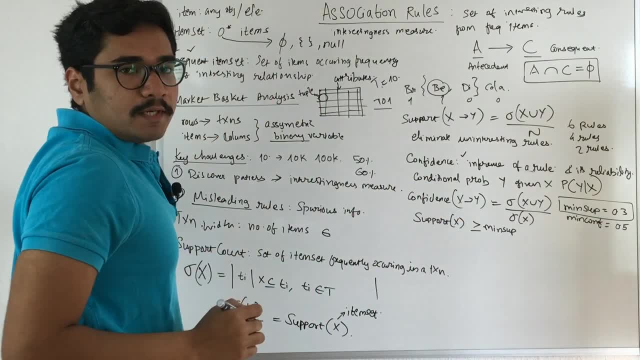 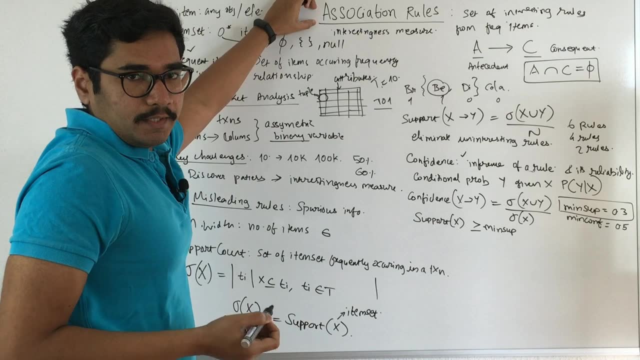 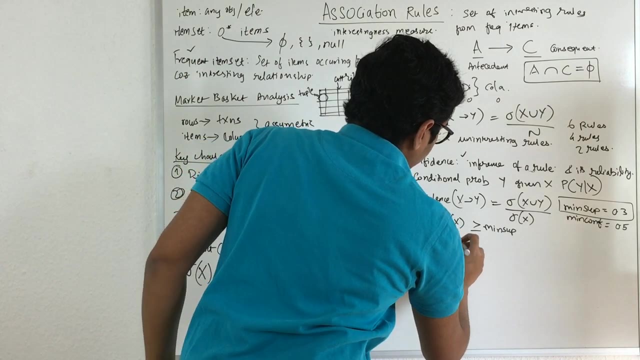 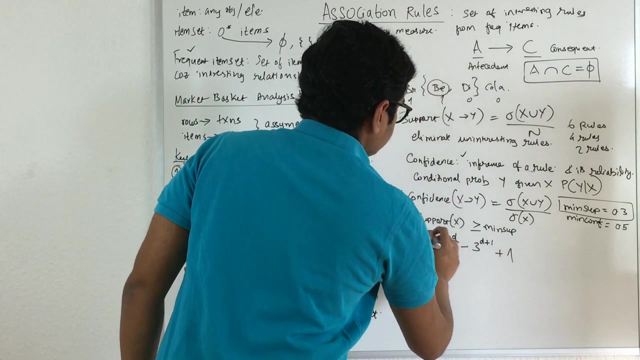 is already defined threshold. You call it as a frequent item set. That is simple. Next, how many number of possible rules That you can derive. so in a brute force approach, say you have a D number of item, so you can derive 2 raised to D minus 3 raised to D plus 1 plus 1 items, So you can derive these many. 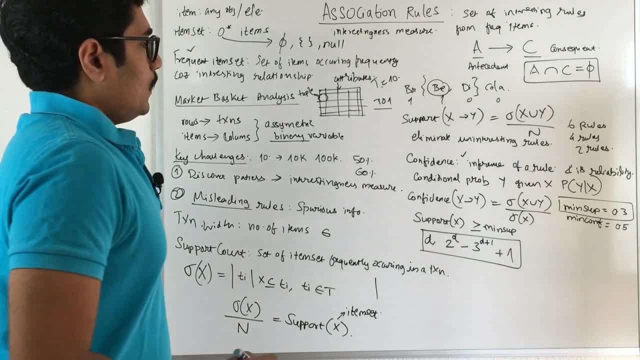 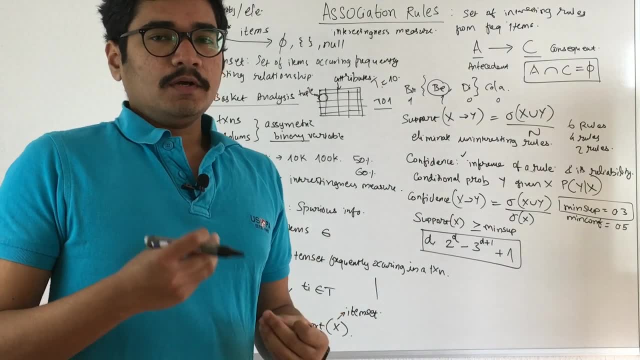 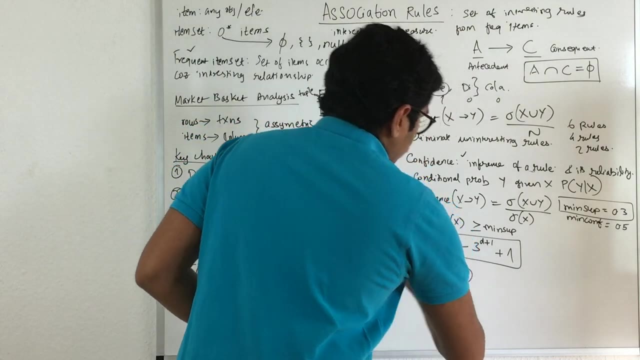 kind of possible rules in a brute force approach. Now how do you eliminate frequent item set? or say you have n number of frequent items are generated. So what are the measures that you can apply in order to reduce this frequent item set generation? So for frequent item set generation you have first to reduce. 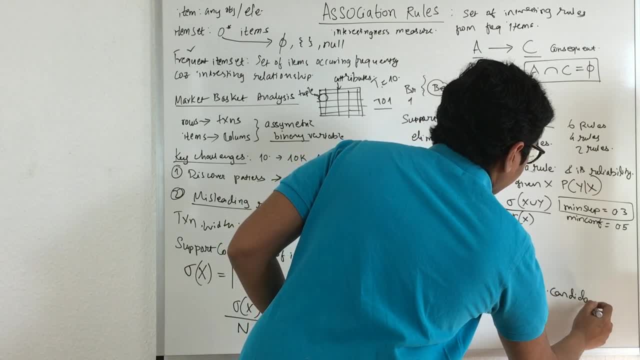 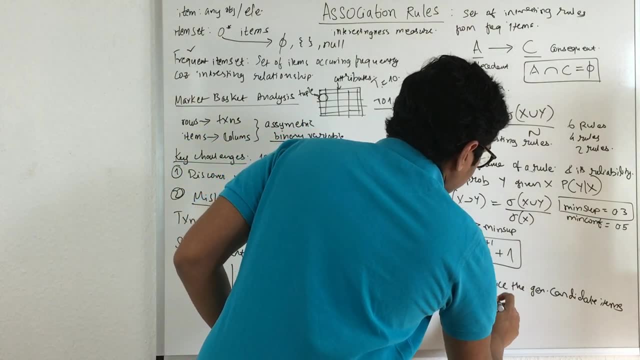 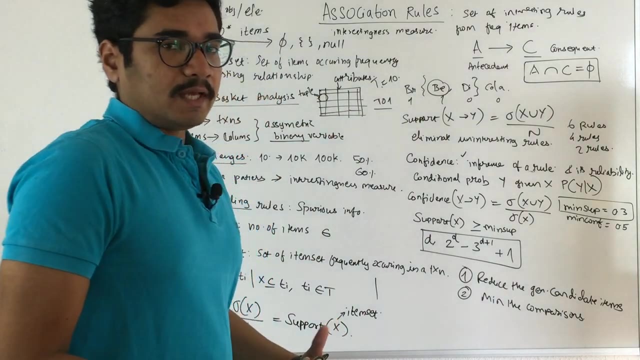 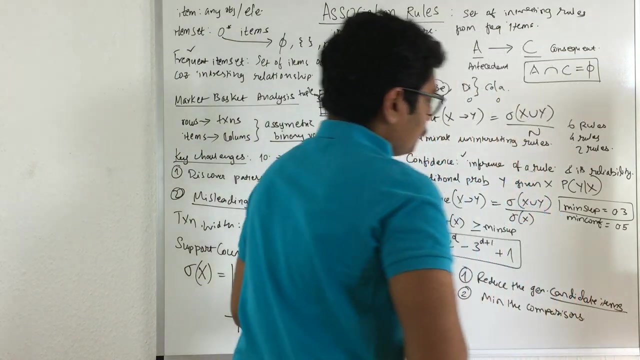 the generation of candidate items. If you generate less candidate items, what you have is you will minimize the comparisons. Now, how this is done, that we'll see in the item set lattice, where this will be more clear. So, just for the time being, you just can understand. 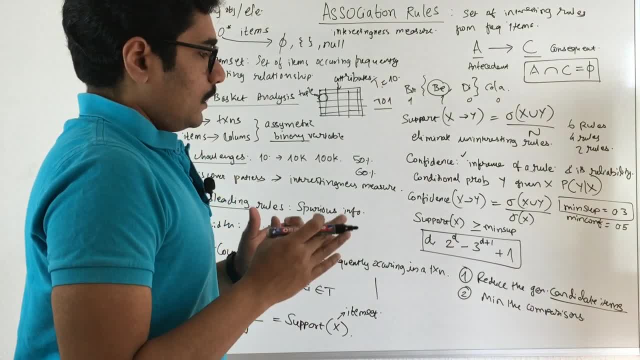 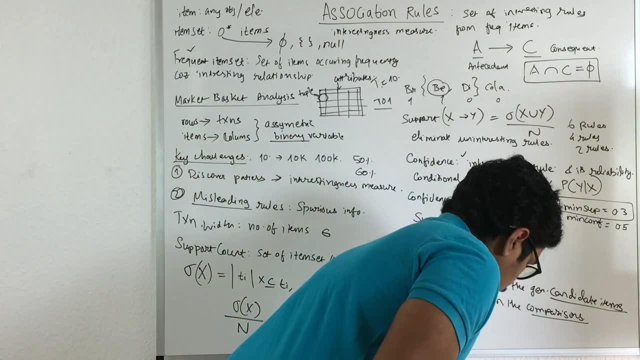 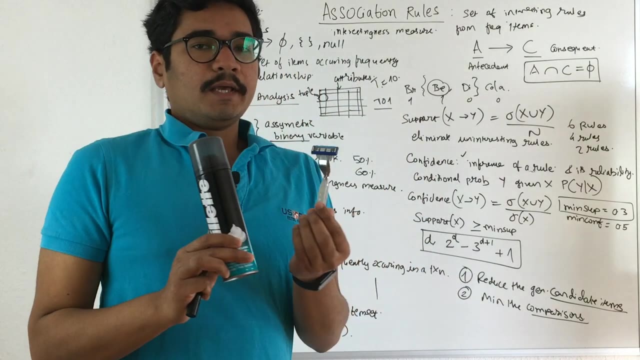 that you need to lesser generate the candidate items and thereby you can minimize the comparisons. So, similarly like this: if you have this shaving cream, then it's also possible that you will buy a razor. So this are frequent items which are occurring together. 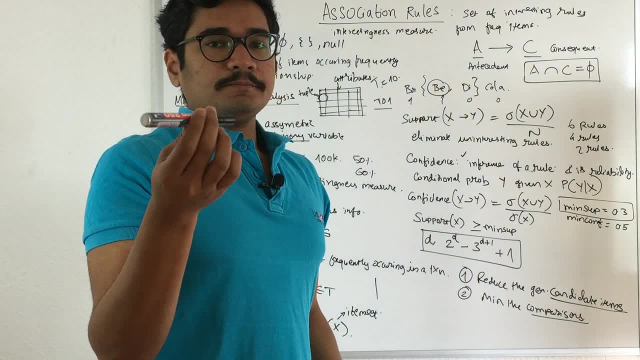 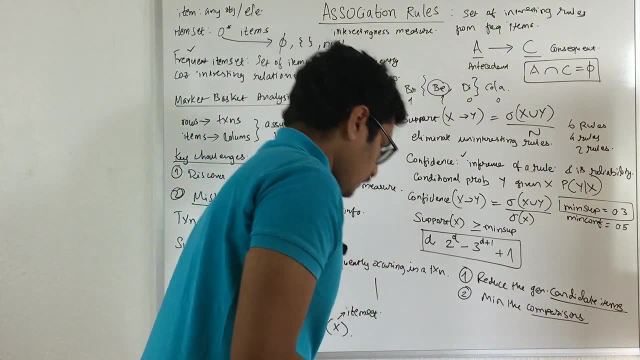 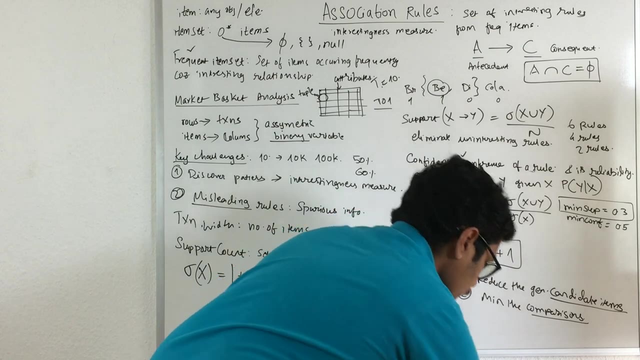 Or if you have this marker itself, you can buy this. you'll also buy this refill station, So these are frequent items occurring together. or you can also buy this duster, So these are frequent items. or with this, you can buy a brush with this shaving cream. 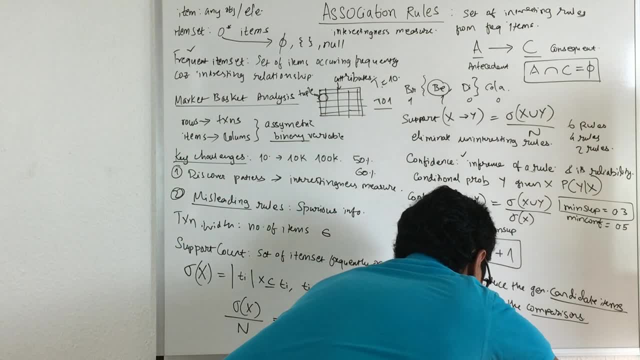 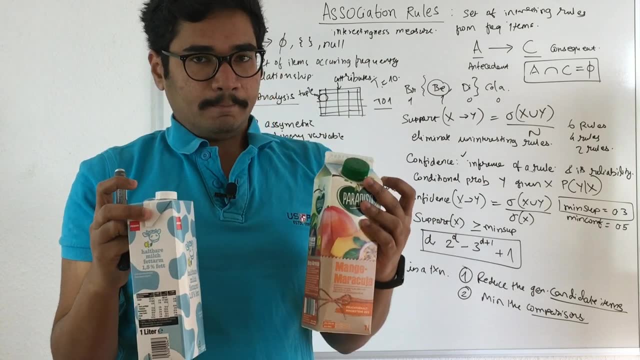 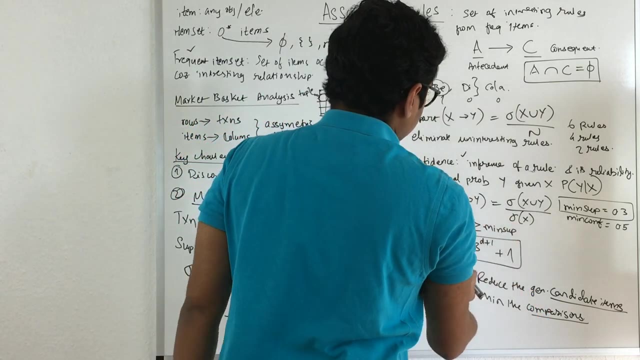 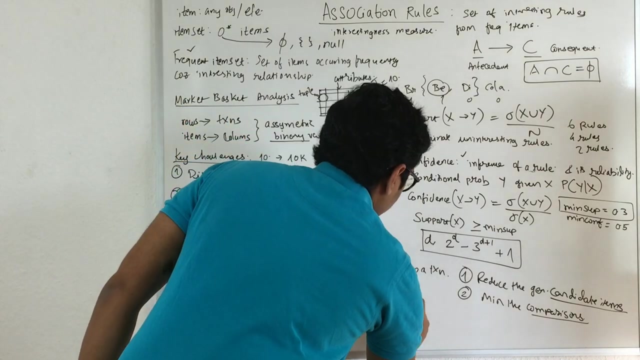 These are frequent items, or milk and juice. So these are frequent items, but it's not that strong. So thereby you define some rule, That is, you have this normal rules. So from that you need to derive some kind of rules which are very strong. 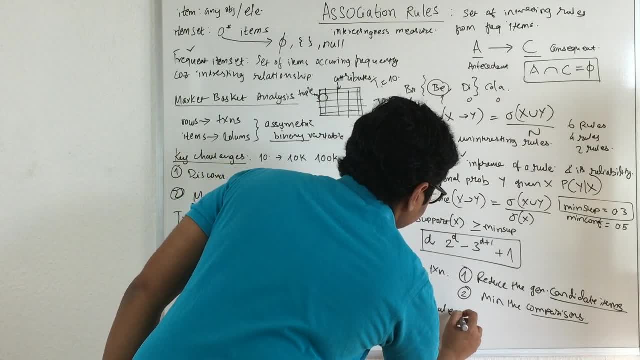 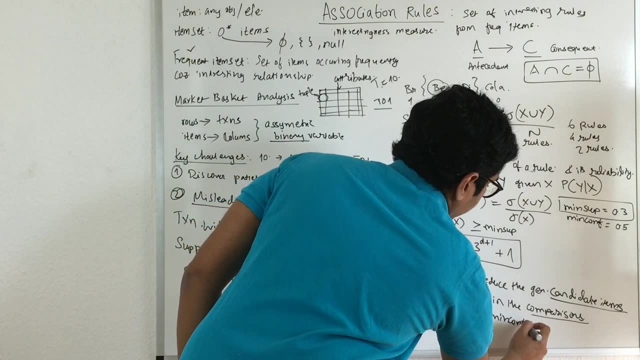 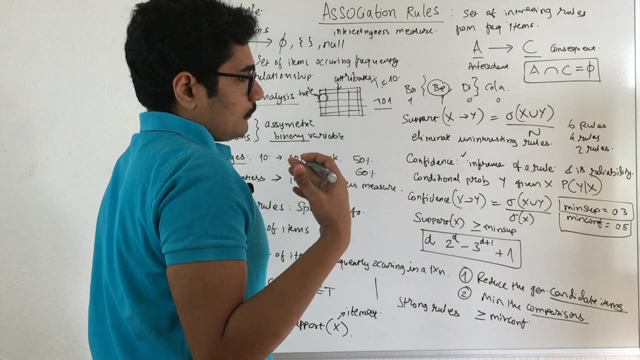 So those are called as strong rules. So how do you determine Strong rules? rules which are greater than or equal to the min confidence which you get from here, which is already defined by the algorithm. So if you have certain kind of rules which are greater than the min confidence, then those 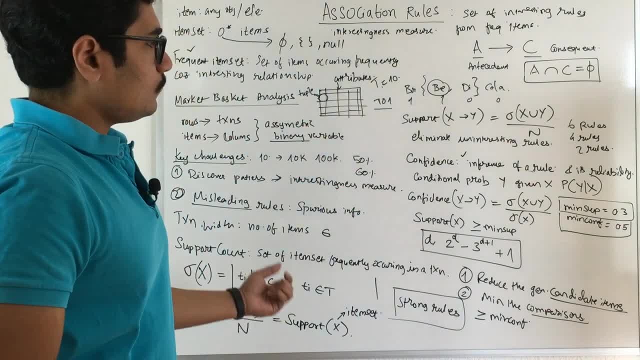 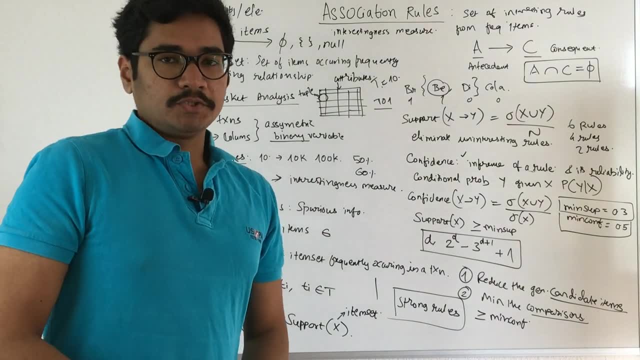 are called as strong rules. So well, that was all regarding some of the basic introductions and terms which are required for Association rules, So hope you guys enjoyed this video. found your educator news video. Please do like, share, comment and for new to channel. Please consider subscribing. Thank you very much for watching this video.